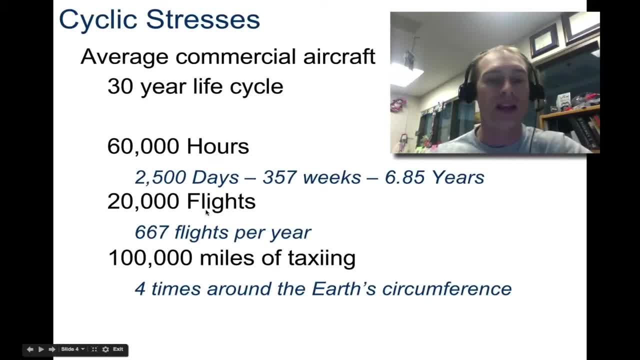 It's a commercial aircraft. It's about 20,000 flights and 100,000 miles of taxiing, which is four times around the circumference. So some interesting facts for you. So this is a total average. maintenance and service cost is usually double the original purchase price. 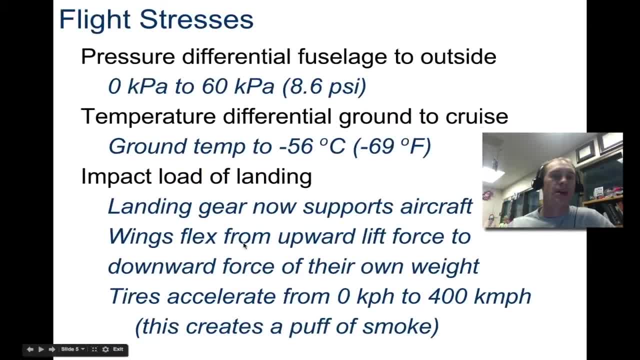 Just to keep it maintained, The flight stresses that it has to overcome are some pressure differential to the fuselage and outside. We took a look at pressure differentials anywhere from 0 kilopascal to 60 kilopascal. Temperature differentials, ground temperature, which is whatever. it is on ground surface that you're at. 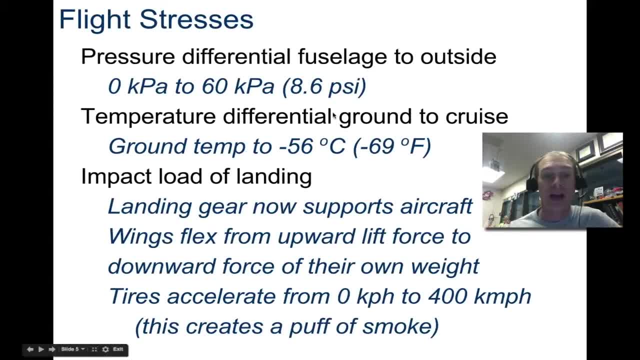 If you're at the equator it might be really hot, Or if you're flying up to Alaska, it may actually be minus 56 Celsius. It's definitely possible. And then you've seen the temperature lapse rate where it can get really really cold as you are flying at high altitudes. 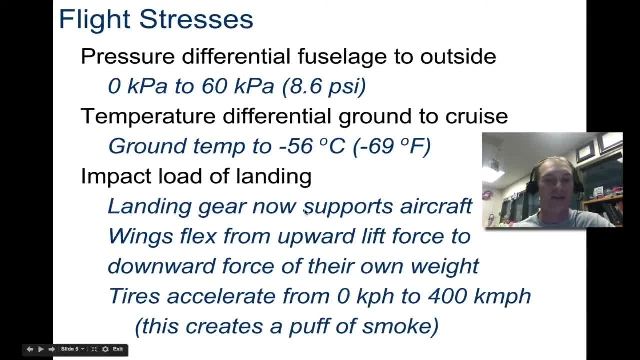 And then there's impact of landing. The landing gear has to support the aircraft, The wings have to flex. When it lands, the wings flex up. So there's a lot of stresses right on the joint from where the wing attaches to the fuselage. 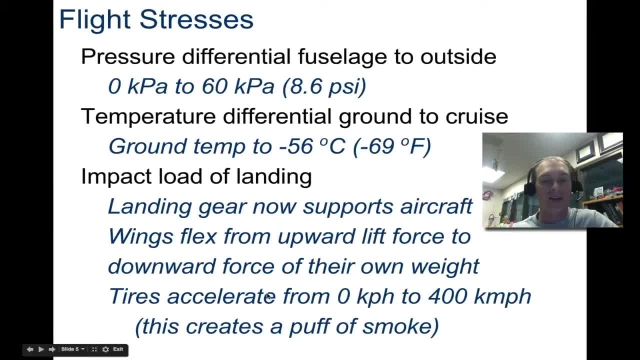 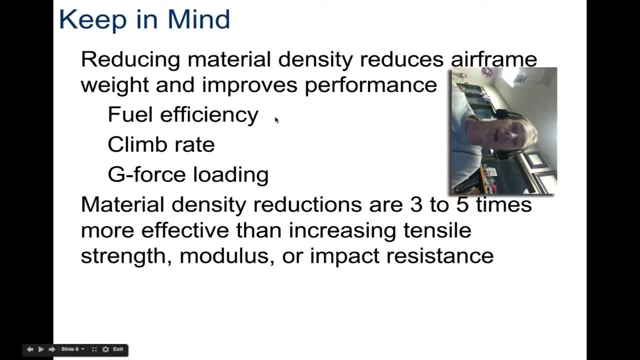 There's also downward force of their own weight, And then the tires are going to accelerate from 0 to about 400 kilometers per hour instantly, which is that little puff of smoke, So they have to be able to handle that. So you need to keep in mind that reducing material density also reduces the airframe weight and improves performance. 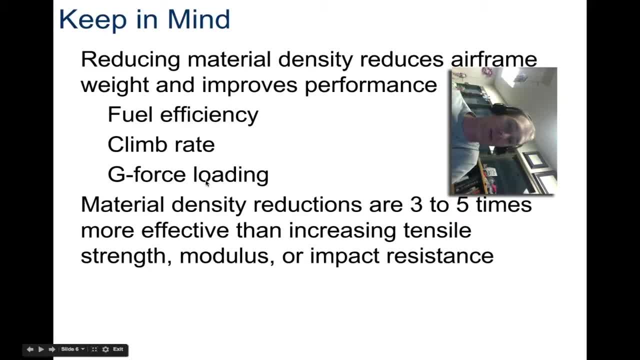 So that improves geoefficiency, climb rate, g-force loading: If you're reducing weight, then things are going to work out better for your aircraft, as long as all other factors are not compromised, As long as all the factors. So you want to keep in mind that reducing material density 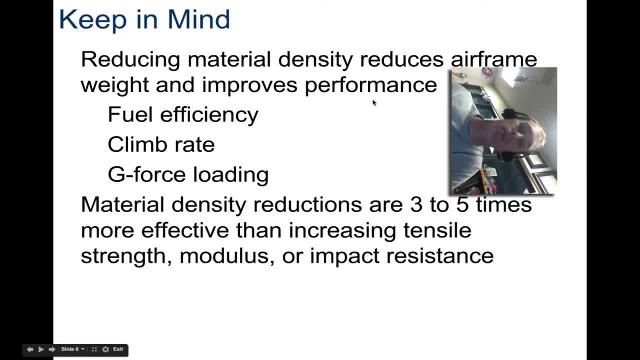 reduces airframe weight and improves performance, which means that you'll have better fuel efficiency, climb rate, g-force loading As long as your weight goes down, then you have less requirements for lift. Material density reductions are 3 to 5 times more effective. 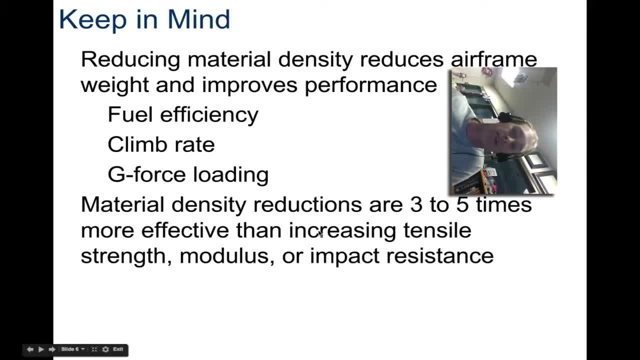 than increasing tensile strength modules or impact resistance. So, rather than making your airplane super, super strong, it actually is more efficient and more effective to make it less dense. So you want to keep in mind that reducing material density makes it less dense. 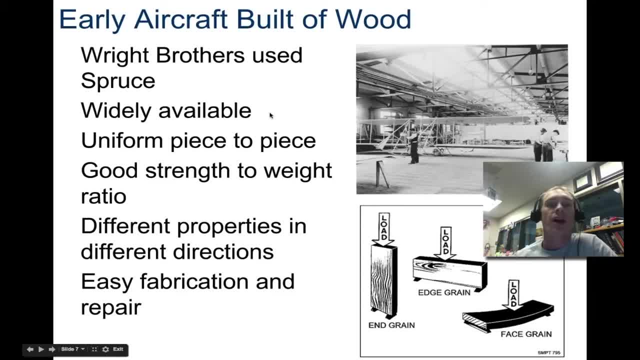 It's 3 to 5 times more effective. So some early aircraft- now we're going to start looking at materials- were just built out of wood and they used spruce. It was widely available. It was relatively uniform from piece to piece. 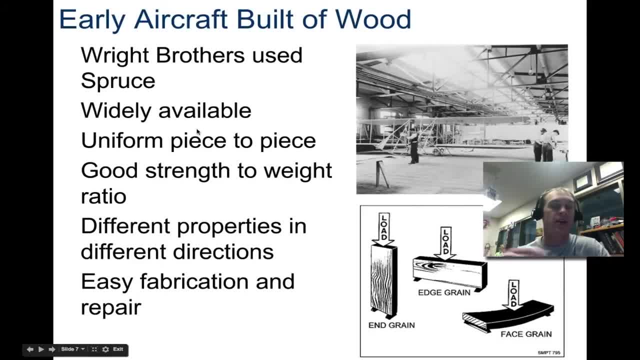 So you didn't have drastic changes in density from one wing to the next, which we saw- some of us saw- with our Balsa gliders- as the density of the wood changed. one side of the aircraft was a little bit heavier. It has a relatively good strength to weight ratio. 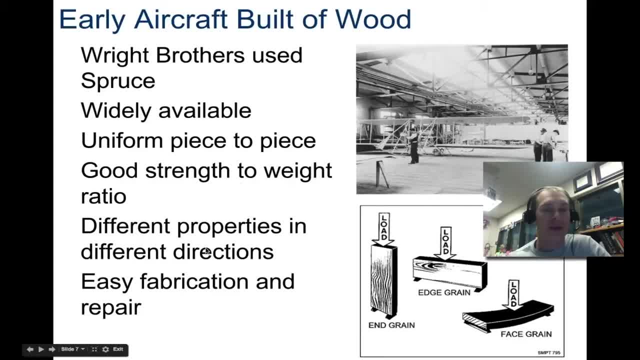 And again there's different properties Depending on the different directions. So if you look at the directions of the wood, if you load it on end grain, it's going to have very different properties than on edge grain or face grain. here And it's relatively easy to repair. 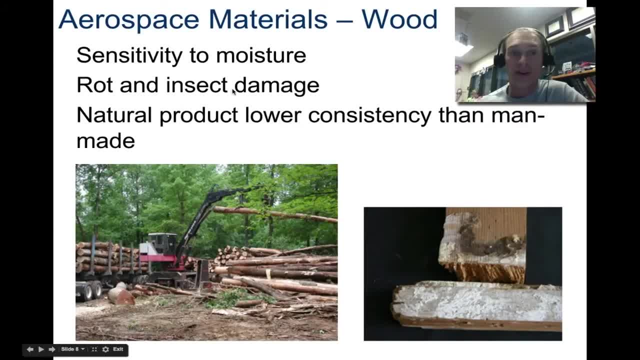 So it seems like the miracle material. However, it is very sensitive to moisture, rot and insect damage And it's a natural product that is lower consistency than a manmade product. So a solid, consistent metal is going to be consistent all the way through. 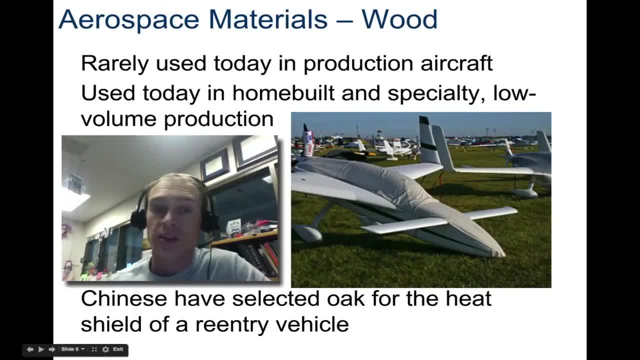 whereas wood is just not going to be. So it's rarely used today because of those things. Some people use them for home-built aircraft, because it's cheap and readily available material. And then, just a neat little fun fact, the Chinese selected oak for the heat shield of a reentry vehicle. 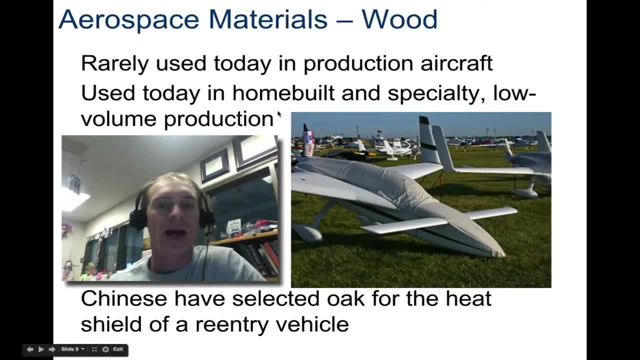 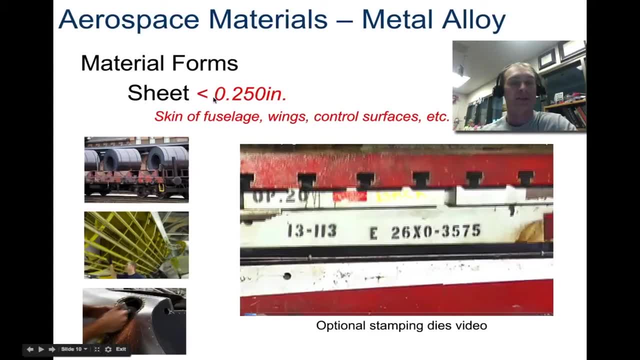 because oak has a really, really high flame point. So here's some different material forms. You may have a sheet material, So something you might want to add. The sheet is less than a quarter inch And this is typically for the skin of the fuselage wings surfaces. 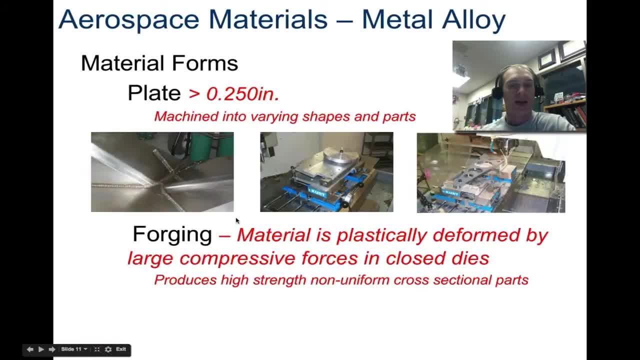 So you have sheet metal usually in these rolls here And you might also have plates, And plates are greater than a quarter inch And these are usually machined into various different parts. So you can see this one has been milled out And that's like plate metal, usually a lot thicker. 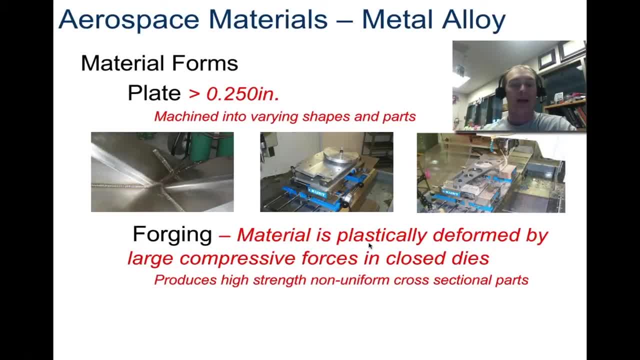 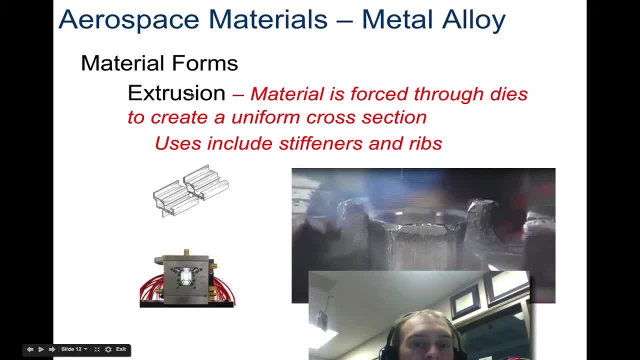 You also may forge it, where it's just plastically formed by compressive forces. You're pushing it into shape, You're using different types of metals, And then there's also extrusion, And we've seen all these videos in the robotics class. 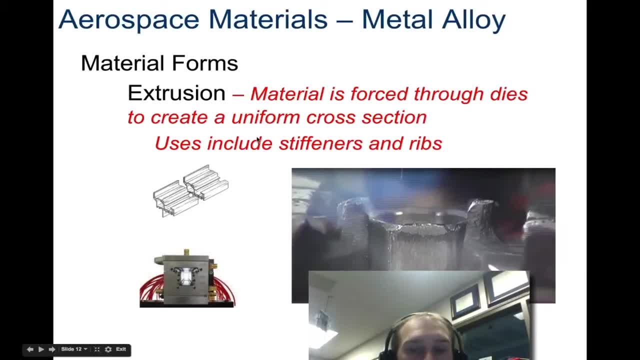 where the material is forced to the dies and it creates a cross section And metals themselves solid. metals themselves can be solidly extruded with enough pressure. Then there's casting. You melt it down, You pour it into a die or some sort of mold. 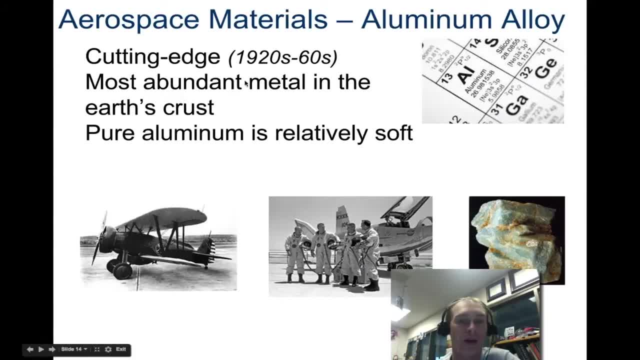 Now we're looking at specific materials, So one of them is aluminum alloy, And this is sort of cutting edge. This is the most abundant metal, So to be able to use aluminum is really important, And in fact, to the point that truck manufacturers are starting to build trucks out of aluminum. 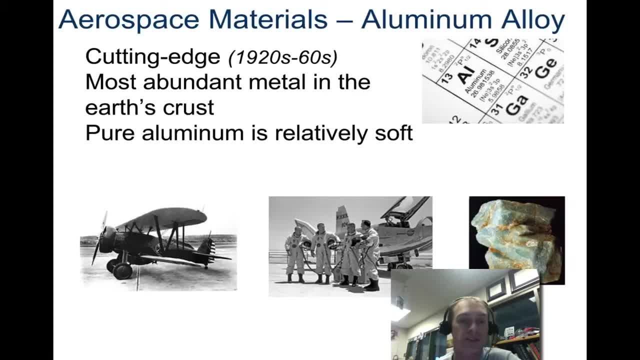 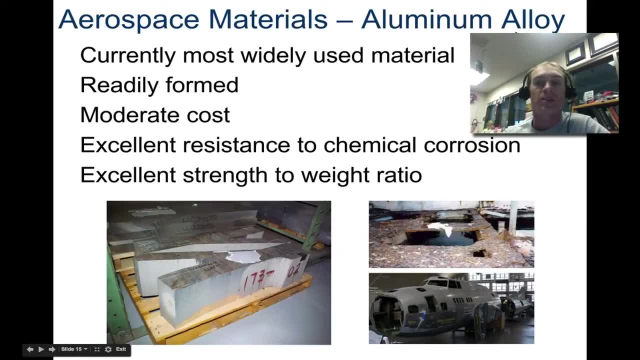 because it can make them a lot lighter and they're really strong, So that improves fuel efficiency. Pure aluminum is relatively soft So they have, through lots of materials testing, realized they needed to make it an alloy, which means mixing different kinds of metals. 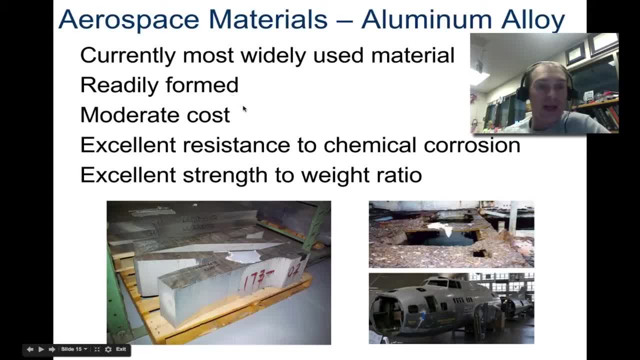 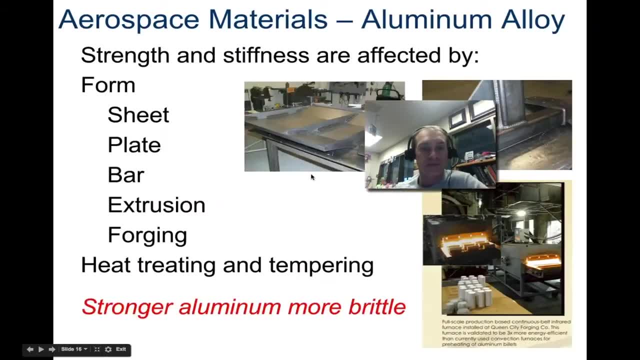 So again, it's relatively or readily formed, It's at a moderate cost And there's good resistance to chemical corrosion and very, very good strength to weight ratio. So strength and stiffness are affected by the form of it: If it's a sheet, a plate, bar, extruded, if it's forged. 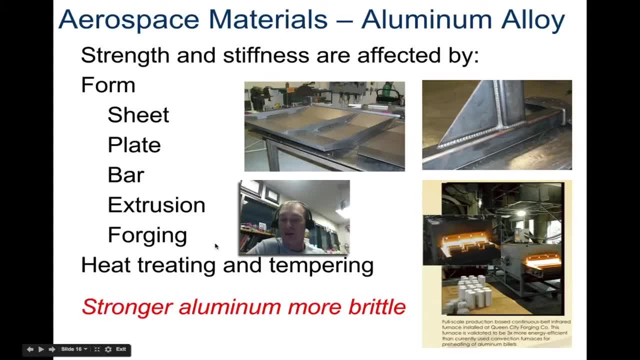 And heat treating and tempering can help affect some of these things too. Stronger aluminum is typically more brittle, And again that just means that it won't deflect very much until it actually fails and snaps altogether. So here's a couple different alloys. 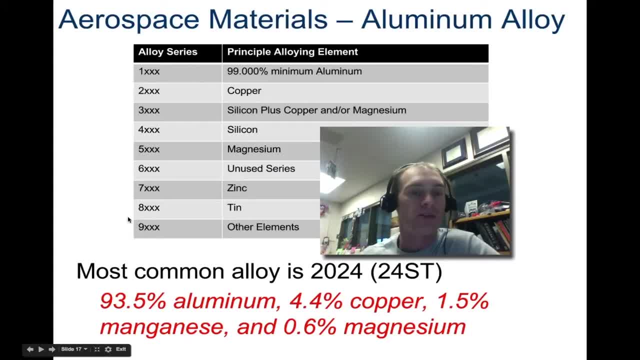 There's actually nine-double of them, And you can see that they're labeled just by these numbers. So if it's a 1000 series, it's 99% pure aluminum. If it's a 2000 series, it has copper in it. 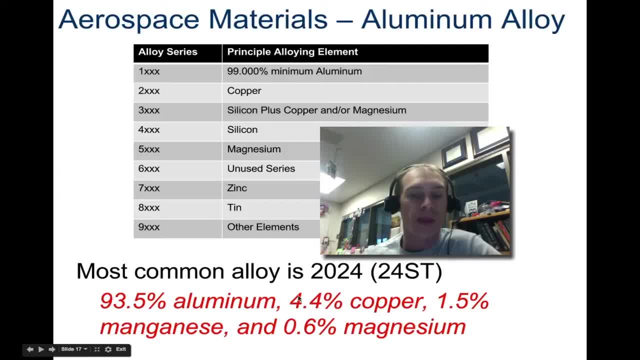 Here's an example of that: The most common alloy is 2024 and it has 4.4% copper. That's the most common secondary element besides aluminum. So these different series will show you what type of aluminum alloy that it is. 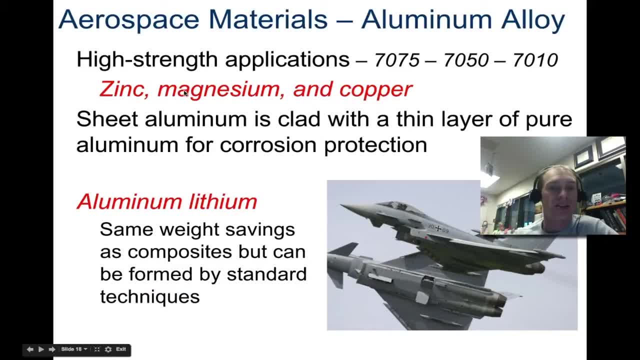 Some really high strength applications are in the 7000 series, And that's using zinc, magnesium and copper. And if sheet aluminum is clad with a thin layer of pure aluminum for corrosion protection, zinc is also used as a corrosion protection Aluminum lithium. this has the same weight savings as composites. 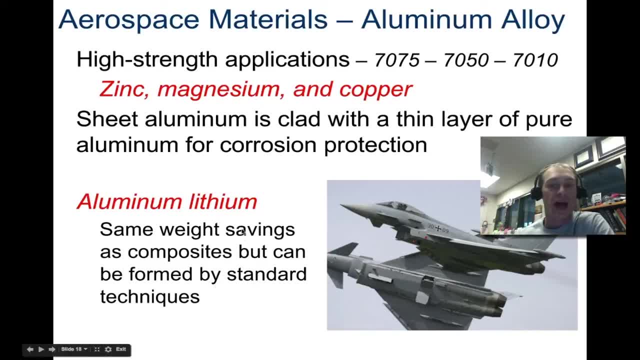 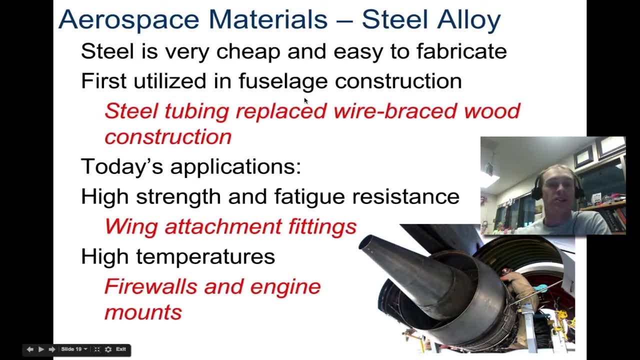 but it can also be formed using standard techniques. So another good alloy Steel moving on is very cheap and easy to fabricate And it's first utilized in fuselage construction. The steel tubing replaced the wooden wire brace constructions And now today they use it as high strength and fatigue resistance. 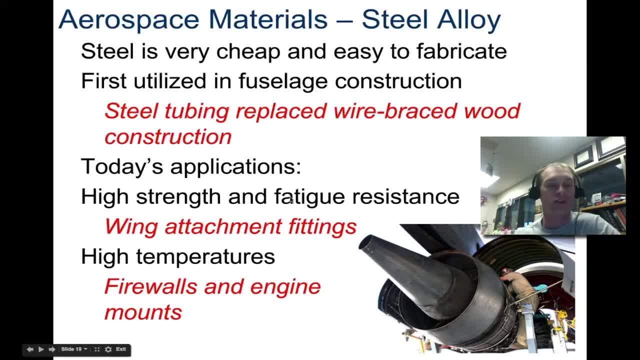 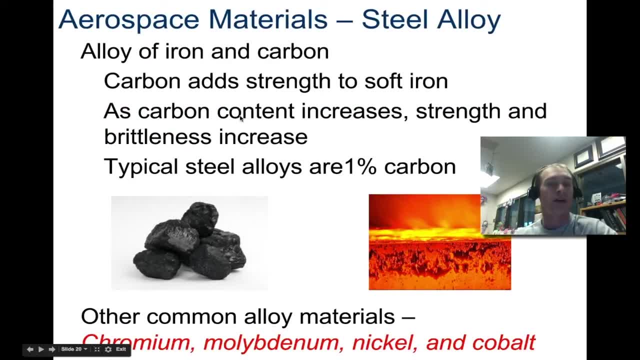 It's for wing attachments. anything where you need something that's extremely strong Steel alloys would be with iron and carbon. So carbon is going to add strength to your soft iron, but it also adds brittleness. So typical steel alloys have 1% carbon. 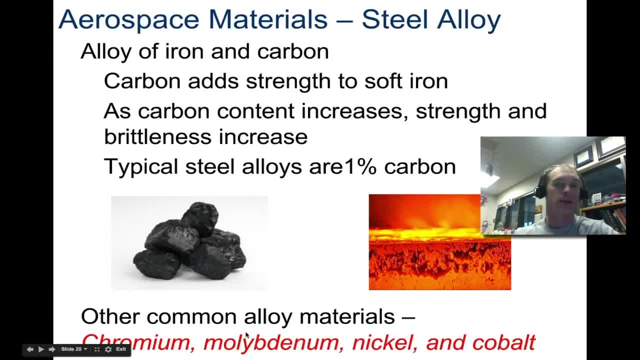 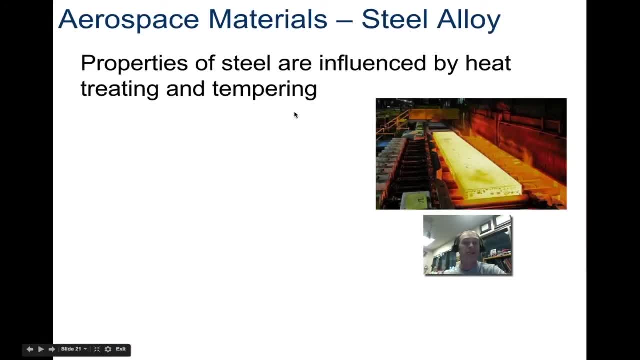 And some other common alloys include chromium, molybdenum, nickel, cobalt. These are just different alloys. These are just different alloys that may be mixed in with it. Steel is influenced by heat, treating and tempering, So you can change its brittleness, its ductility. 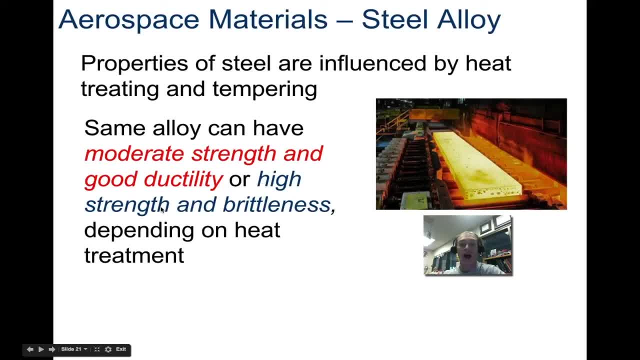 So some of them can have moderate strength and good ductility or high strength, and they're very, very brittle. They don't flex at all. So you may want a product that gives that flexes before it breaks, just given what the conditions that it's going to be in. 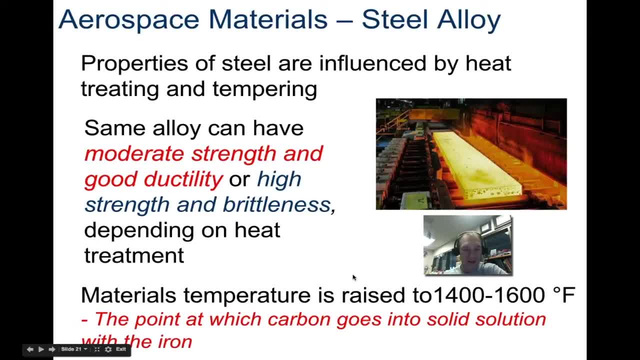 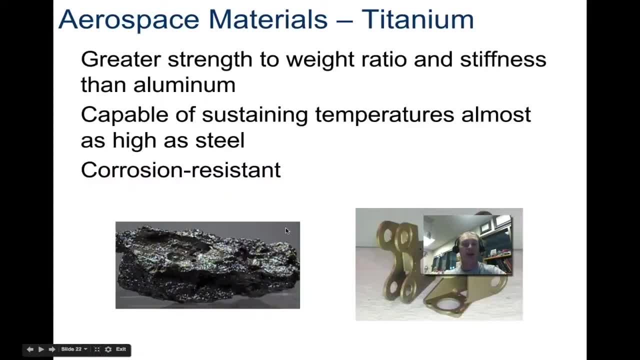 And then materials temperature is raised from 14 to 1600 degrees Fahrenheit, And that's the point where carbon goes into a solid solution with the iron. So you really have to get hot to make that alloy. Then, moving on to titanium, it has an even greater strength to weight ratio. 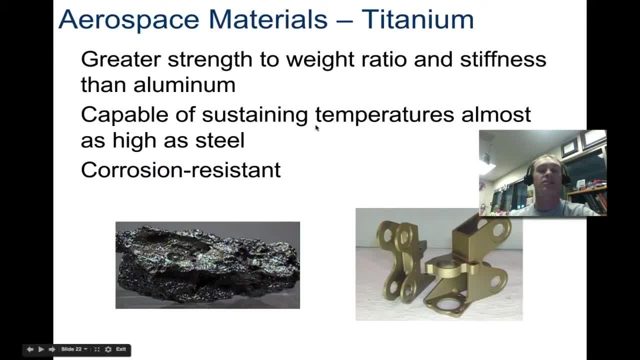 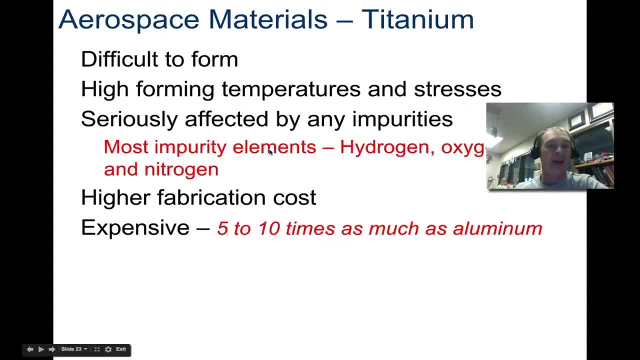 and stiffness than aluminum, And it can sustain extremely high temperatures like that of steel. So that was kind of steel's benefit. Now, titanium gives you a little bit of both, But the downside is it's difficult to form. It has really high forming temperatures and stresses. 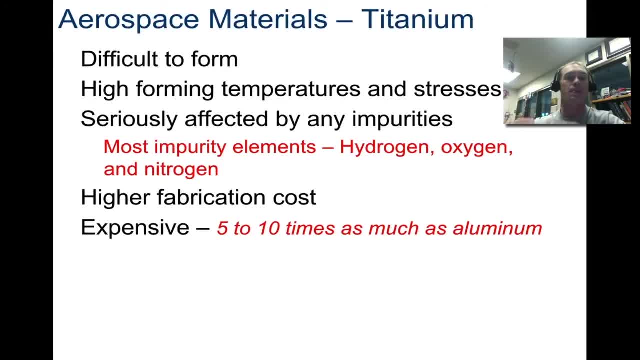 So if you want to extrude it or form it or shape it, you've got to get really hot and you have to have a lot of pressure involved. It's also very, very expensive, which is why it's only used in only applications that need this super great strength to weight ratio. 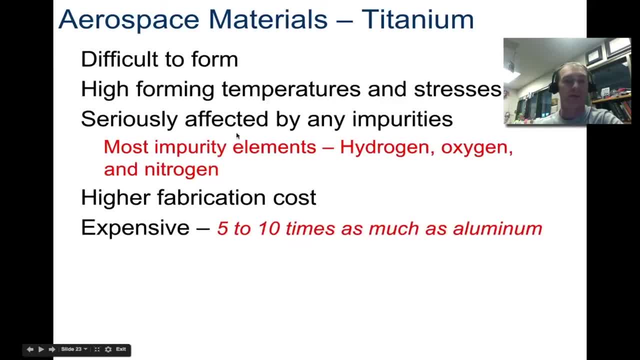 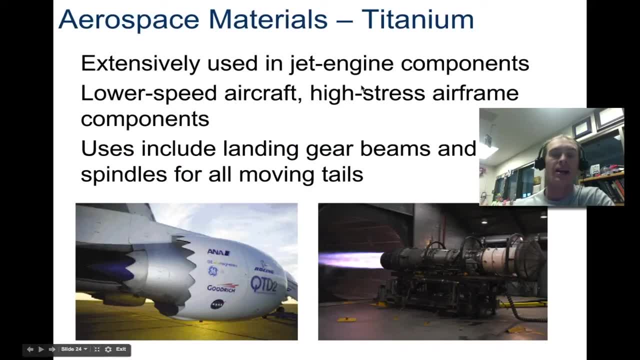 and to be able to sustain high temperatures like that of steel. So, moving on, that's why it's extensively used in jet engine components, that extremely high temperature and really a lot of pressure in there. Also, in lower air spirit aircraft it's for high stress airframe. 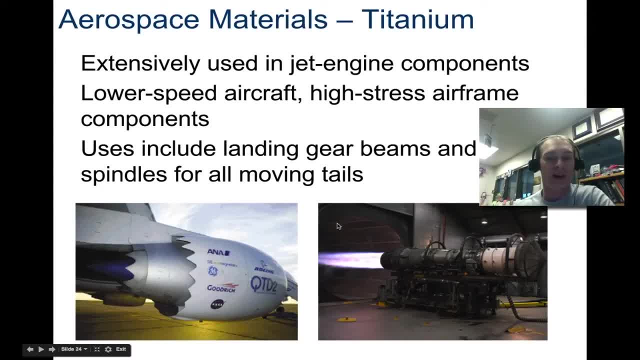 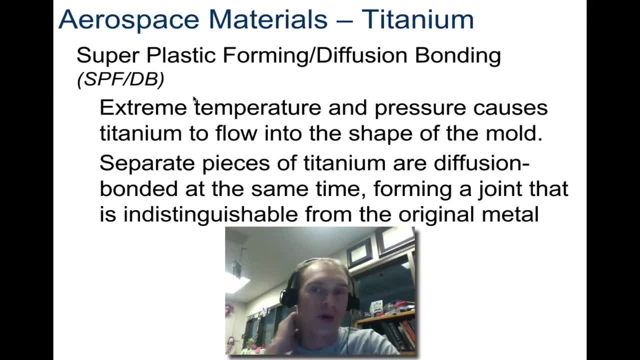 And it's also used in landing gear beams, because that's a part that is undergoing a lot of stress. You don't want that to fail. The way that they actually form this is they use this super plastic forming or diffusion bonding, And they take extreme pressure and temperature and press it together. 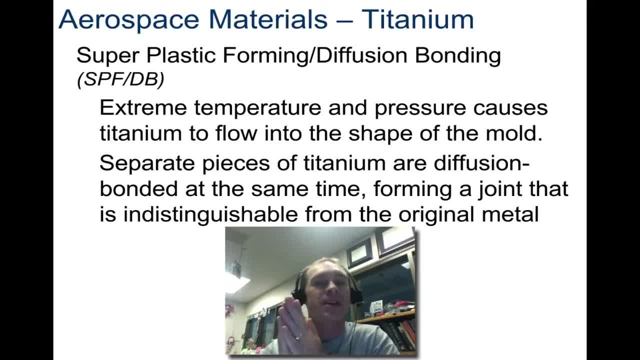 And in doing so it sort of melts or fuses them together. So there actually is no seam when the two pieces are together, It's completely indistinguishable, And that's what it's saying down here. You can't tell where the joint is when you do diffusion bonding. 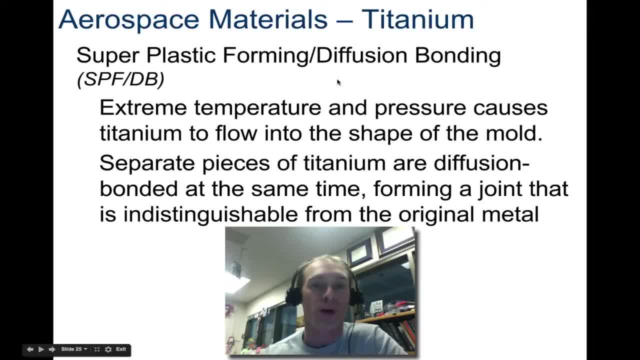 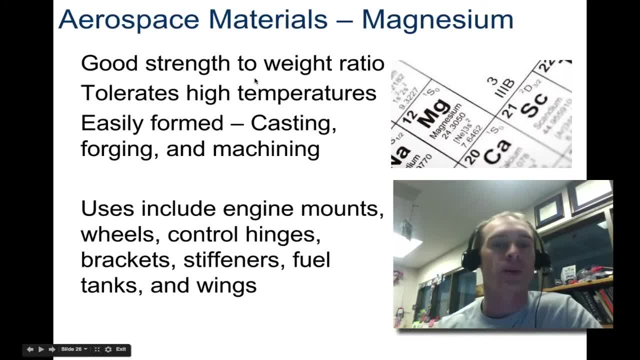 So if you're curious about it, Google it. It's kind of a cool bonding process. Another material has great or good- sorry- strength to weight ratio. It tolerates high temperatures, But if you get too high then it is flammable, which we'll talk about in a second. 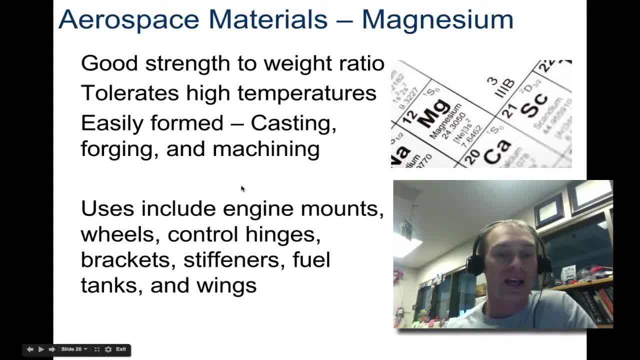 It's easily formed by casting, forging or machining, So it's used for engine machining: Engine mounts, wheels, hinges, brackets. Engine mounts is kind of an interesting thing. When the engine's really hot. wouldn't there be an issue of it exploding? 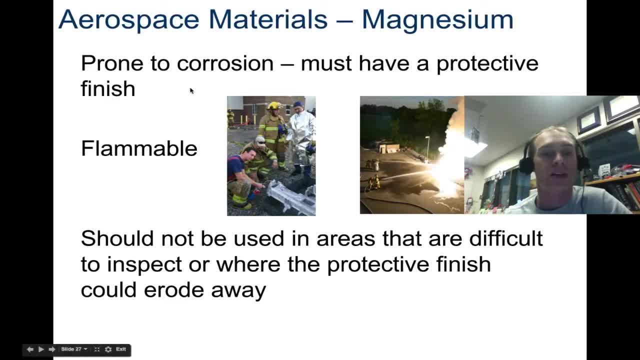 Well. so since it is prone to corrosion, it has to have protective finish. So a lot of times it will be coated on the outside, maybe zinc coated, so that it doesn't just catch on fire. That is usually bad on an aircraft. 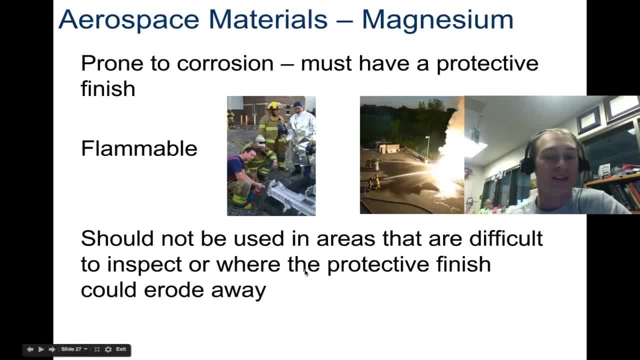 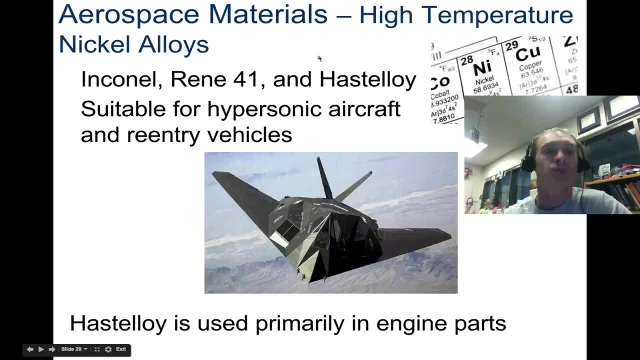 So you don't want to put it in an area that is difficult to inspect. So you might miss that some of the protective finish has eroded away, Because then you're putting it in an area that is difficult to inspect And the plane is going to blow up. 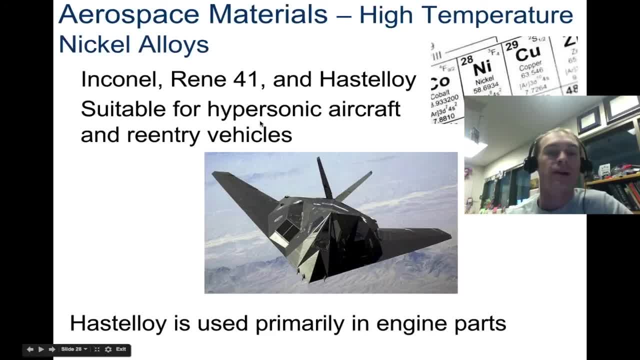 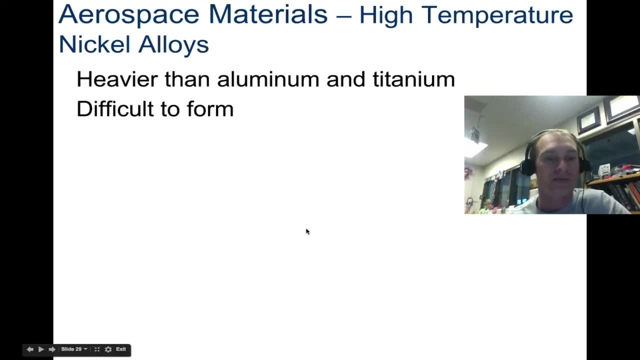 Really high temperature nickel alloys. Here's a few of them, And these are great for hypersonic aircraft that are getting extremely fast, So they have a lot of drag And they get really, really hot through the atmosphere, And this one haste alloy is primarily used in these engine parts. 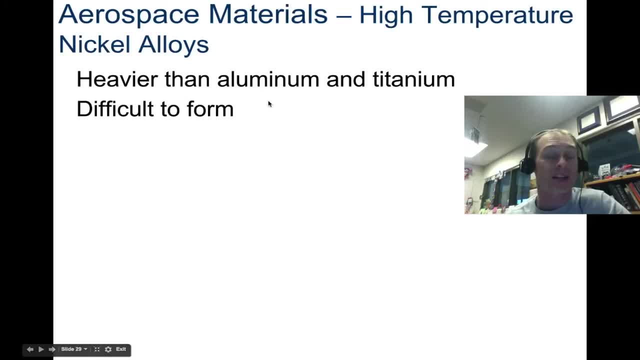 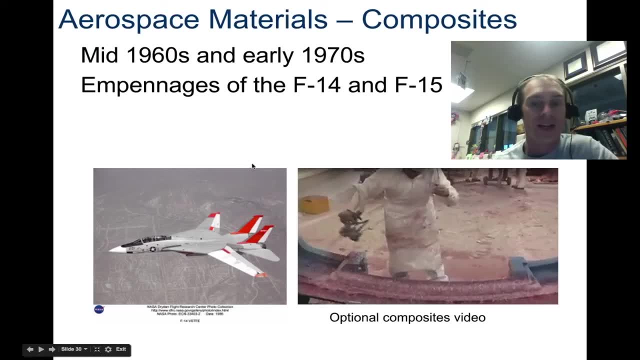 So, again, some of these are heavier than aluminum or titanium, Difficult to form, But they're really great at heat resistance. So now let's look at some composites. Composites are using two different materials together, Where each one separately might not be very strong. 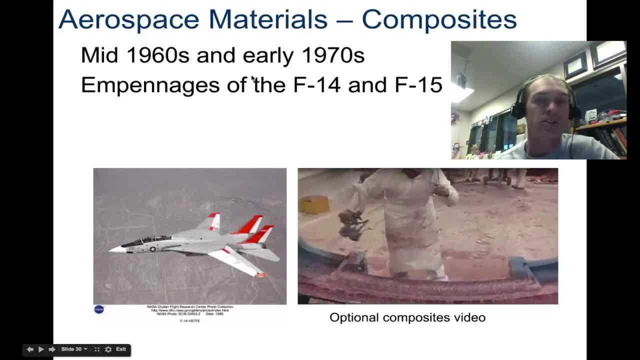 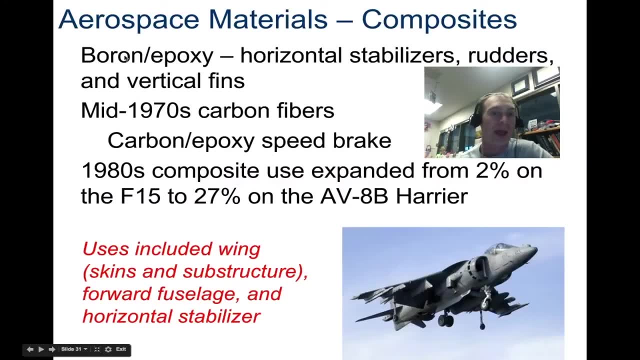 But together they're extremely strong And first used in the 60s and 70s- Part of the empennage, this back part here of the F-14 and 15. And used of an epoxy And then some type of material.